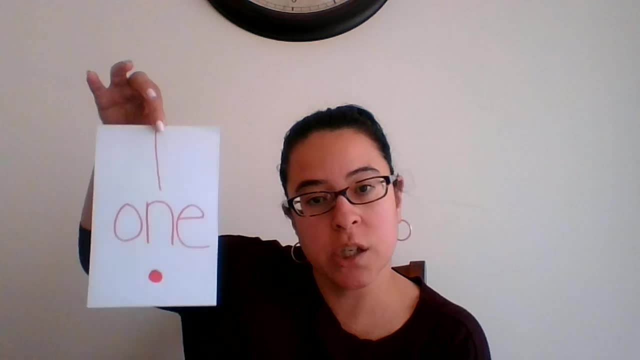 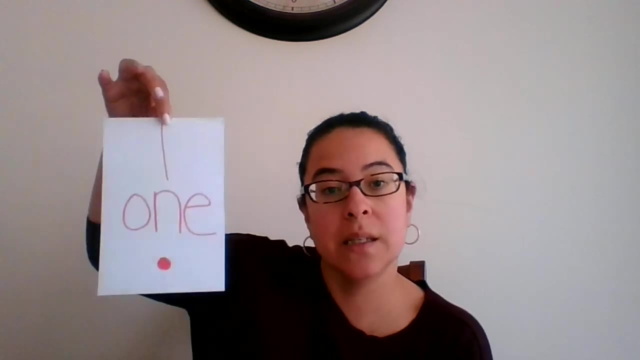 For this activity. Ms Yolanda is going to do the cards from one to five. At home, your mommies and daddies or family members can help you make these cards up to ten, But we're going to do these cards from one to five. 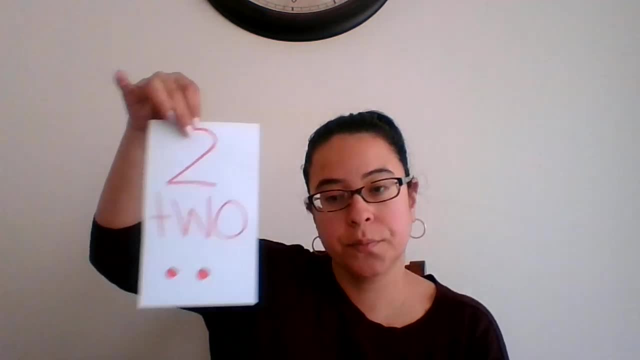 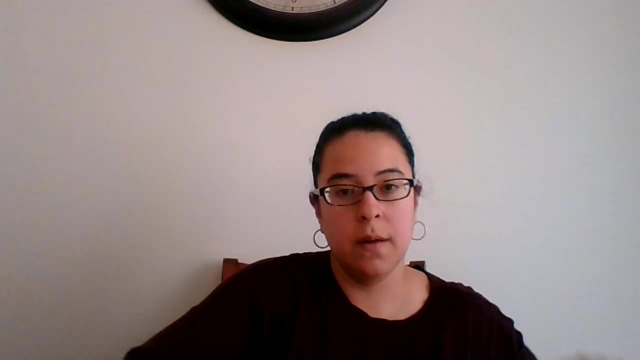 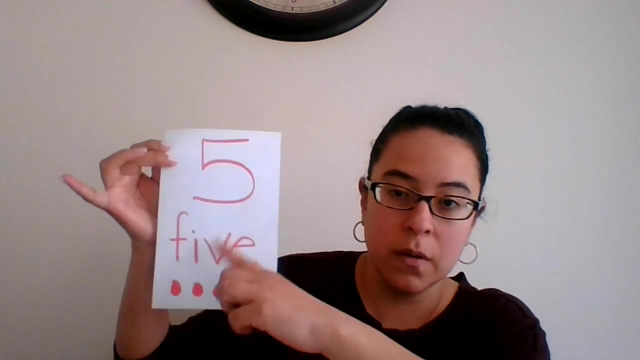 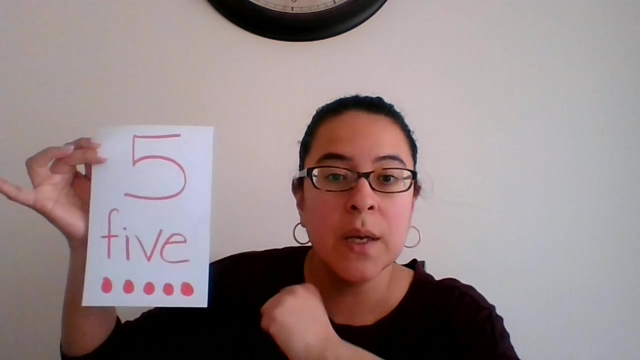 So we have one, two, three, four and five. As you can see, the card has a number, the number name And some dots. So children can be on different levels And it's easier for some to recognize either the number. 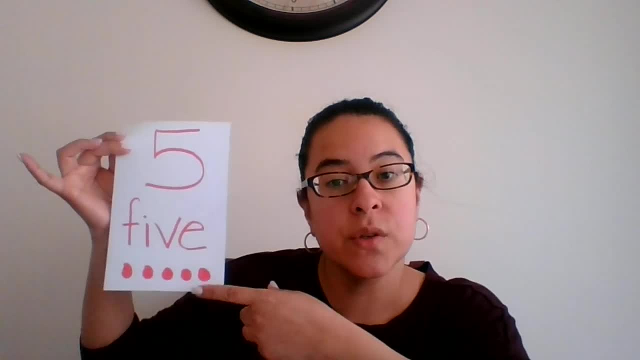 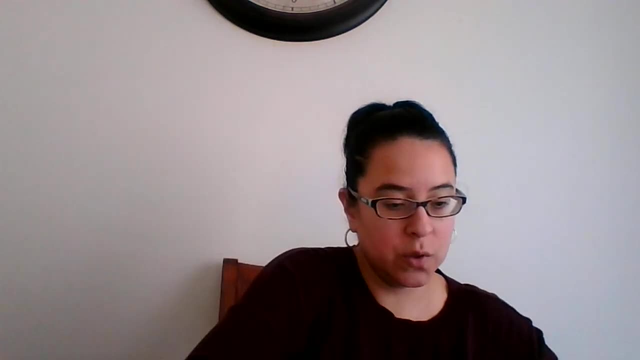 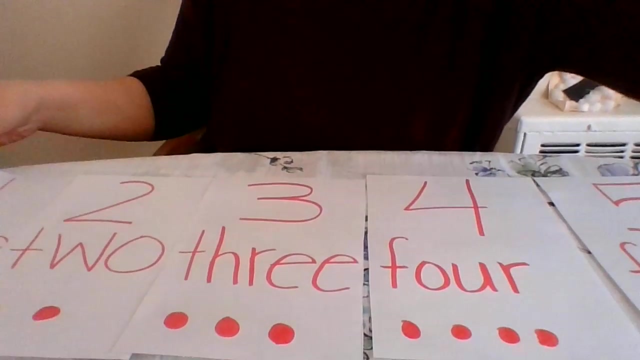 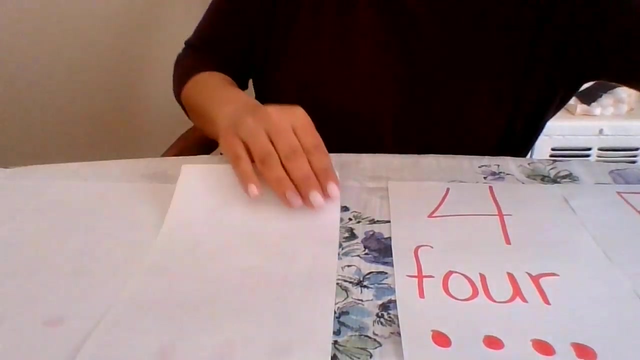 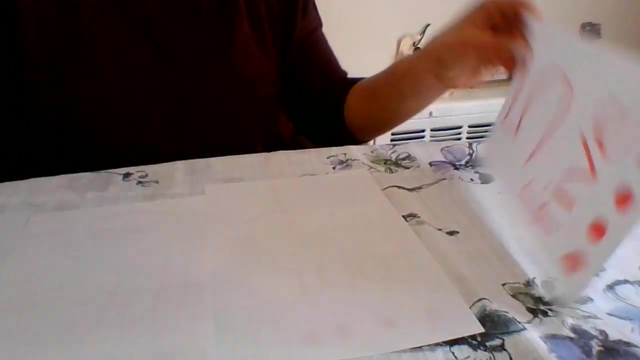 Some can recognize the number name Or others can do it by counting the dots, Okay, So we're going to flip these cards over, Okay, and we're going to keep them in numerical order. So it's one, two, three, four and five, okay. 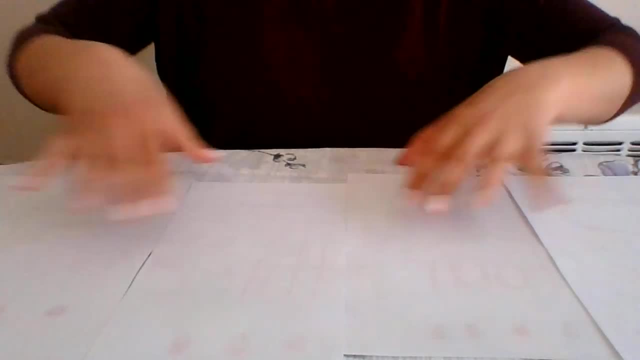 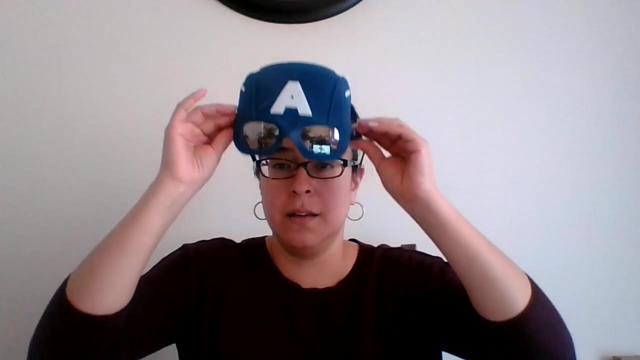 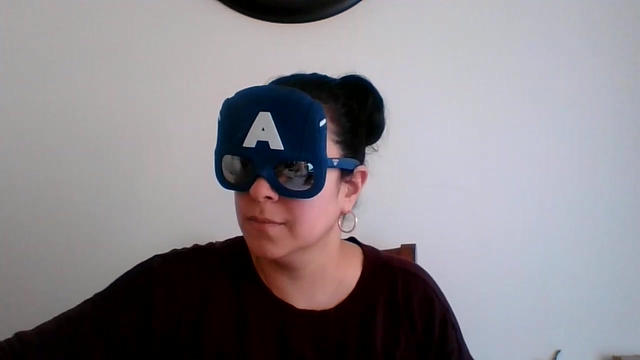 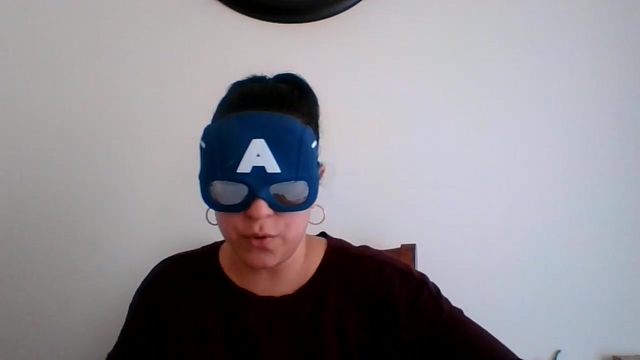 So we have these cards in numerical order from one to five. We're going to grab our x-ray vision glasses- okay, I borrowed mine- And we are going to Play a game and we're going to try and figure out what number is under these cards. okay, 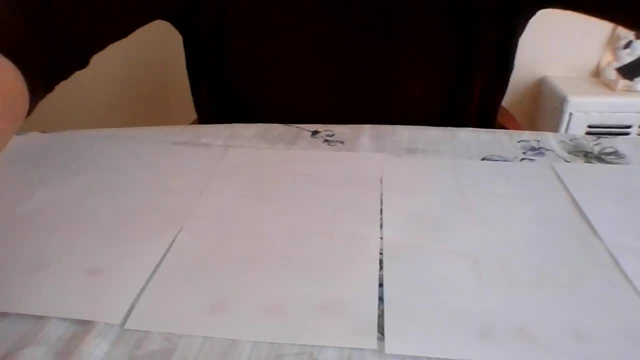 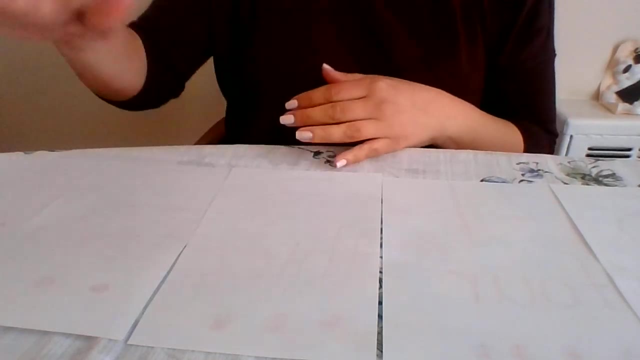 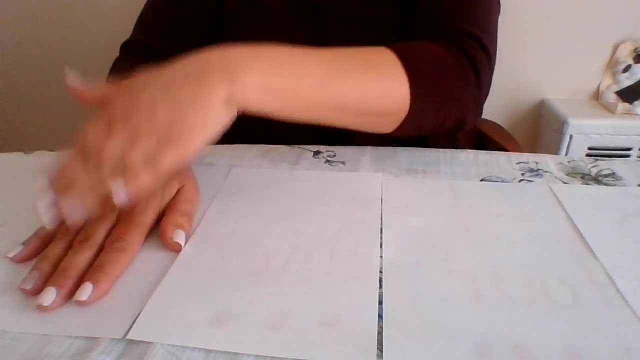 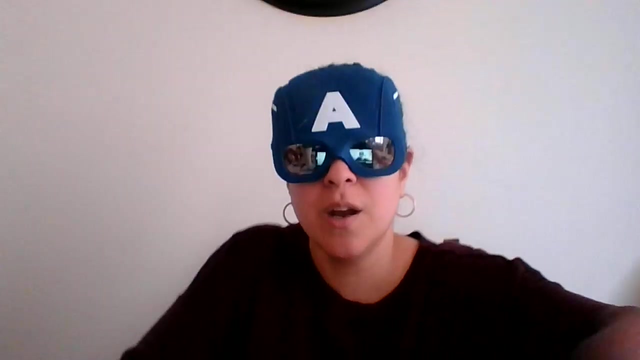 So I'm going to pick. let's see this card. all right, Now let's use our x-ray vision glasses And try to figure out what number is under this card. Let's think about it. What number do you think? 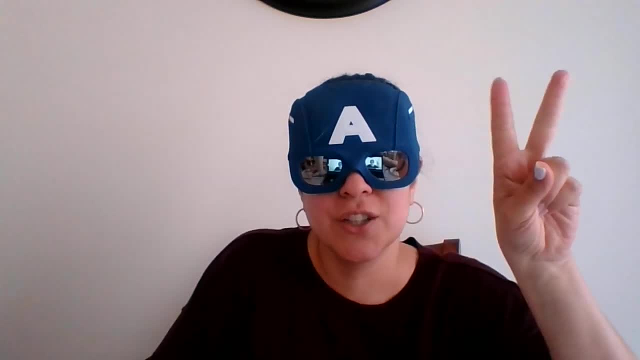 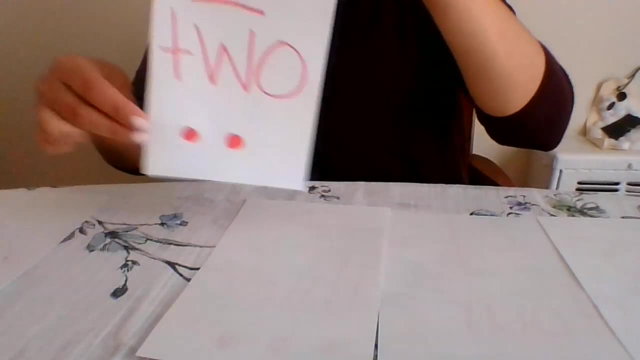 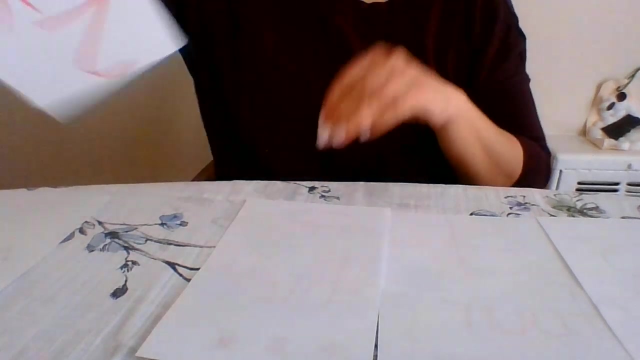 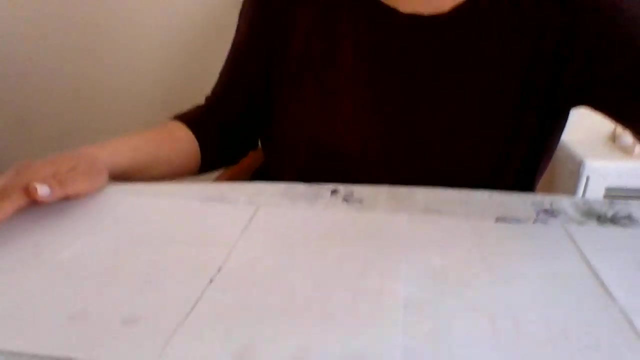 Yes, Number two. That's right, Number two. Let's see, Let's flip it over And it is the number two. And how do we know this? Yes, That's right, because you counted. you counted, You started from number. you may have started from here, from the beginning, from number. 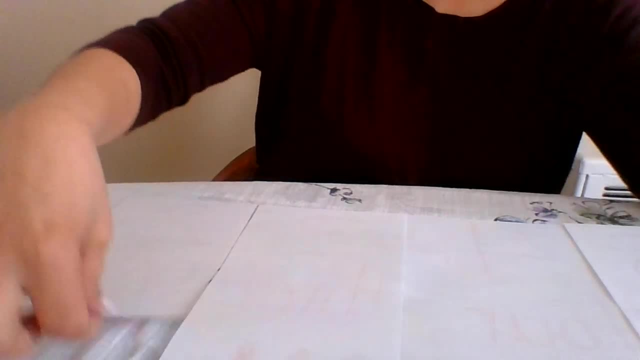 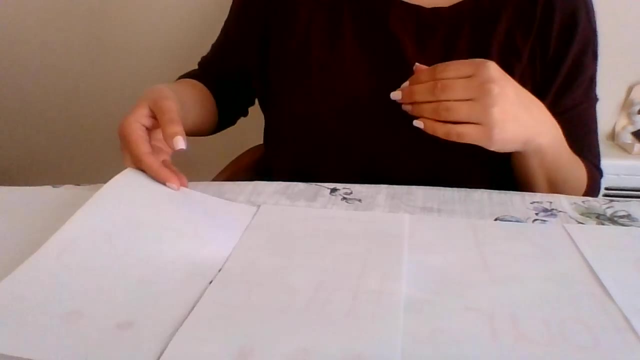 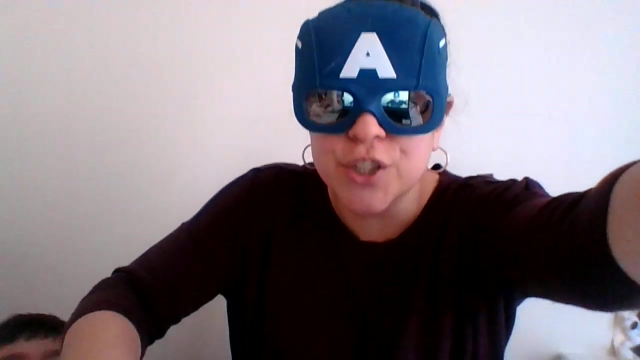 one right, So one, two Very good boys and girls. All right, let's flip this card over and we're going to choose another one. Are we ready? Put those x-ray vision glasses on? We're going to choose another number. 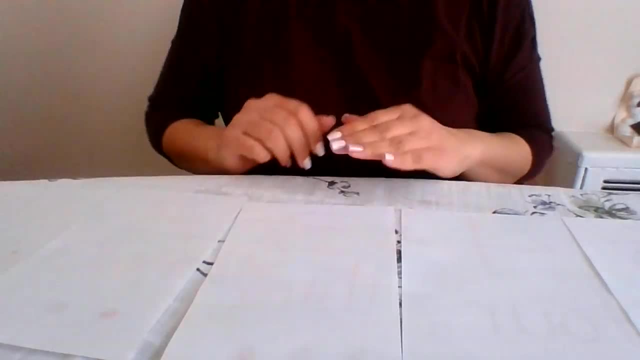 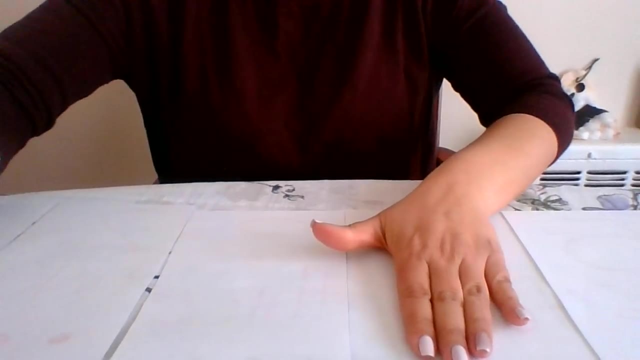 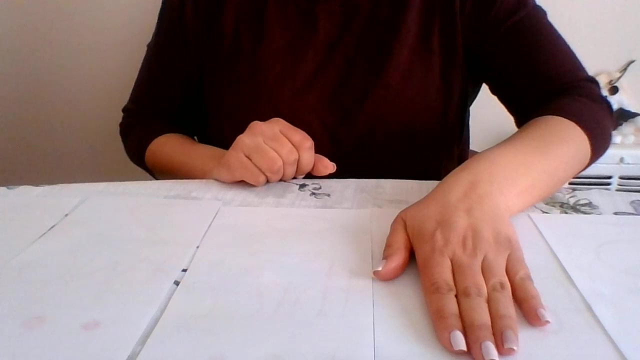 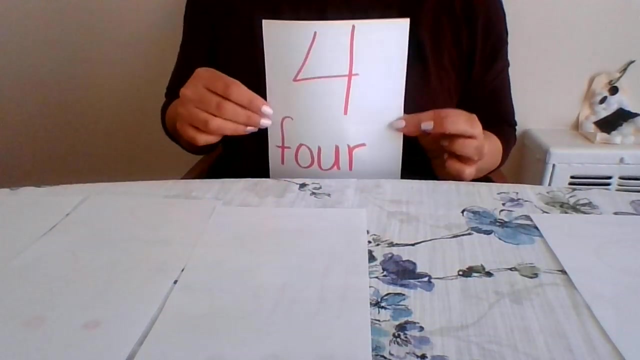 And here we go. I'm going to choose this card. What number do you think is under this card? Let's see. Did you say four? Let's see, Yes, Four. And how do we know that? How do we know that? 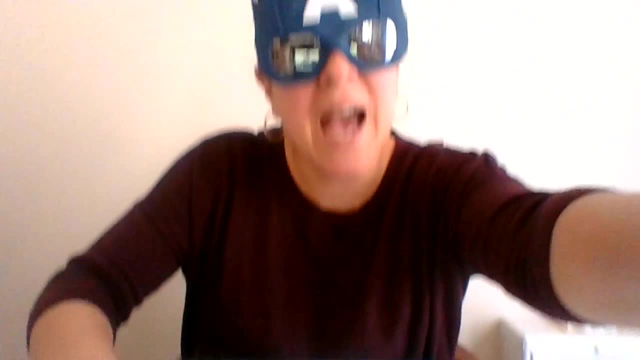 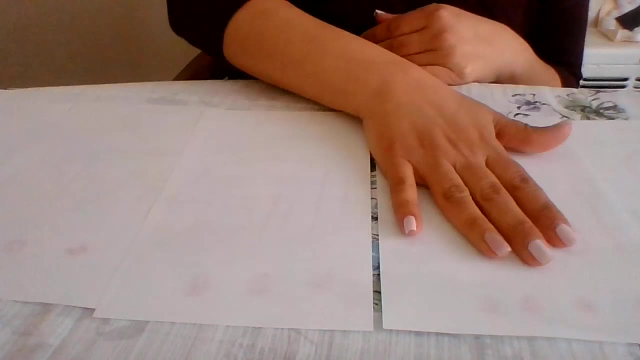 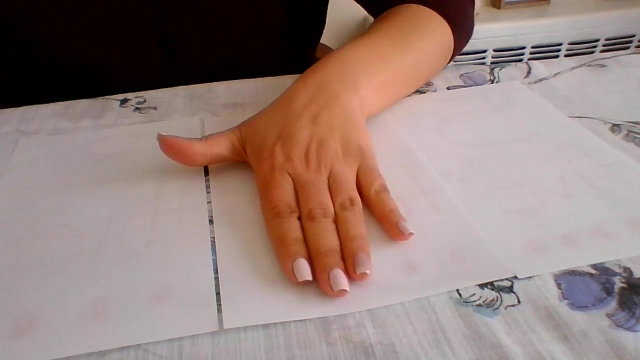 Because you counted. Very good, Let's count together: One, two, three, four. Excellent. What's another way that we can figure out that this is the number four? Yes, Good, We can count backwards: Five, four. 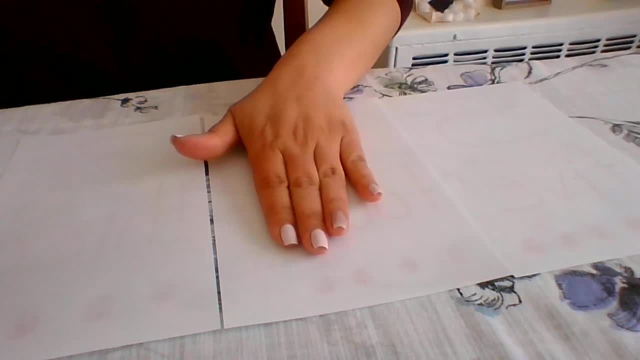 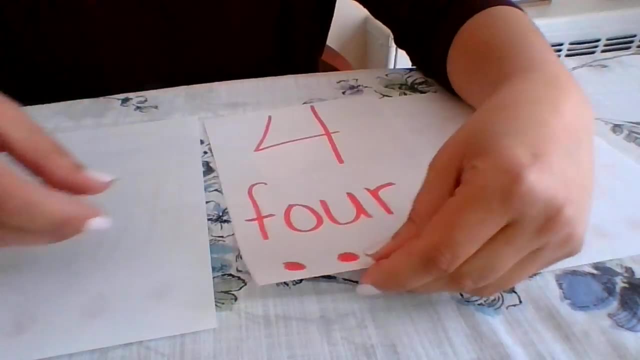 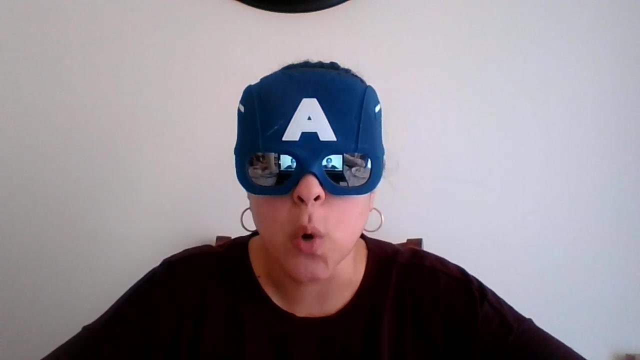 We know this is five, Five, four. We know this is five, And then this is four. Very good, Okay, Excellent, All right. so, boys and girls, you can play this game at home with your family members or your older brothers and sisters. 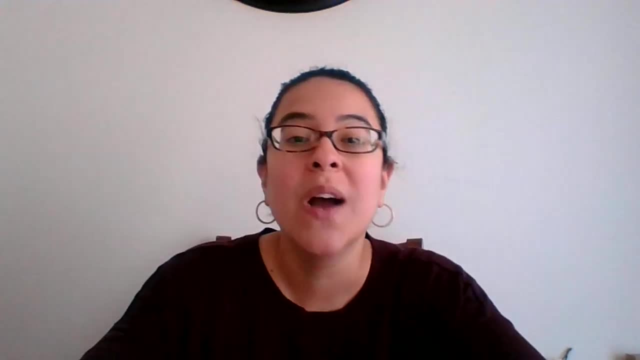 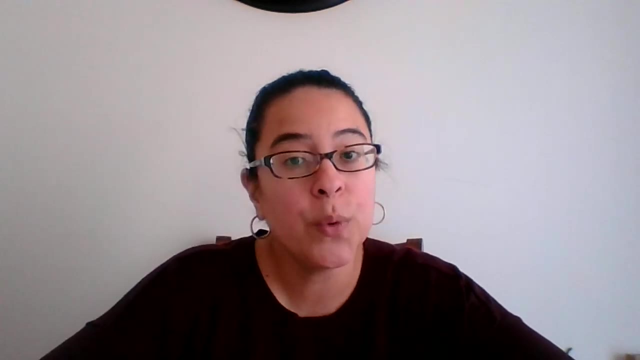 And we can do this up to the number ten. Okay, We can make these cards up to number ten, So I hope you had fun And this will be a fun game to play later With your family members, and your older brothers and sisters can help you as well. 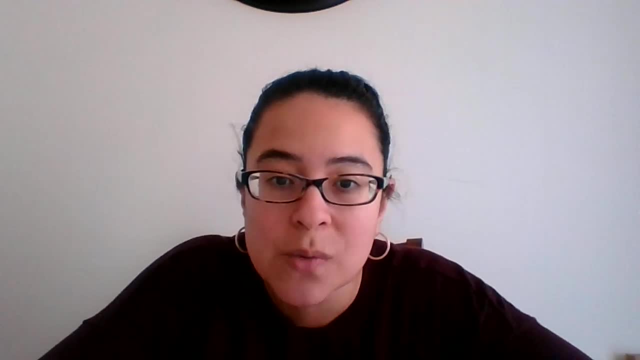 Okay, See you later. Bye.